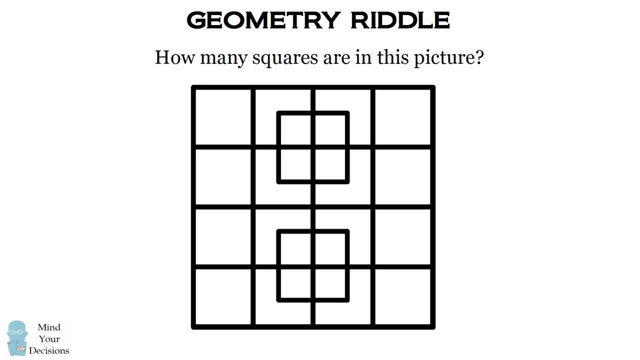 Hi, this is Presh Talwalkar. How many squares are in this picture? Give this problem a try and, when you're ready, keep watching the video for the solution. One way to solve this problem is by counting the number of squares very carefully. 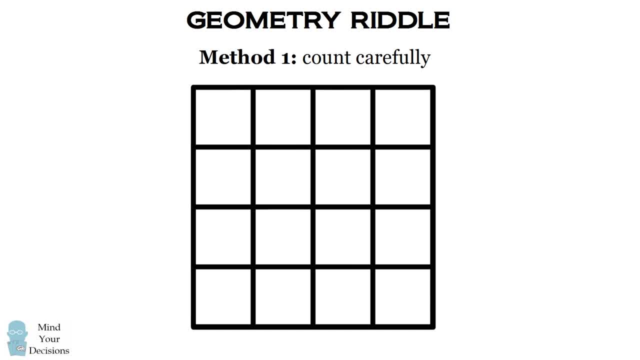 We'll remove the two squares that are in the middle, to be left with a 4x4 grid. Now we'll count the number of squares of different sizes. There's exactly one square that's 4x4, that's the big square. 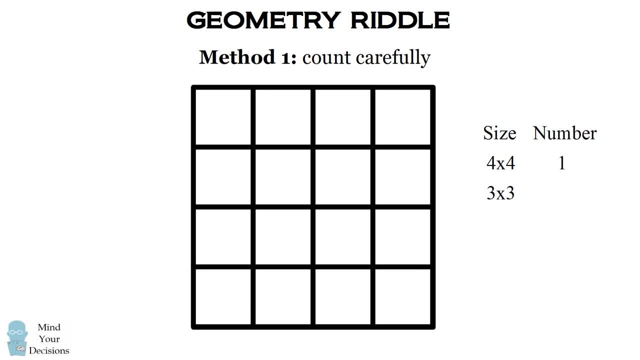 And then we'll count down the number of squares of smaller sizes. The number of 3x3 squares can be found that they're two squares per row and we can count this for two different rows. So there are two times two or four different squares of 3x3 size. How many 2x2 squares are there? In a given row we can place three 2x2 squares And there are three different rows that we can create squares, so there will be three times three, which is nine 2x2 squares. 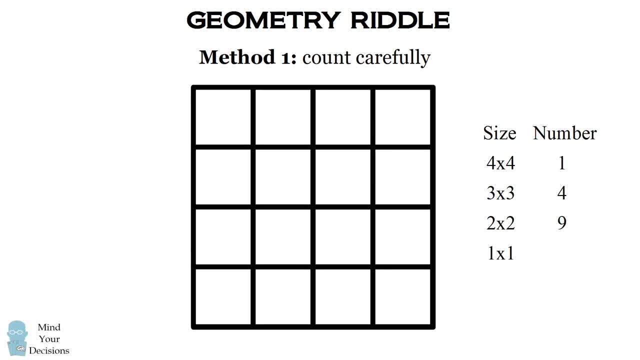 Finally, we count the number of 1x1 squares. There are four different squares in a row and we're going to have four different rows that we can do this. So there will be four times four, which equals 16 1x1 squares. 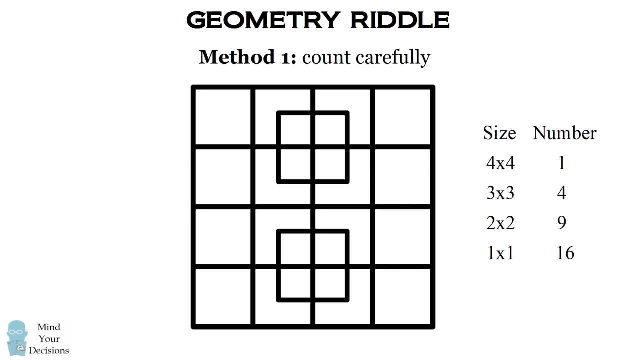 We now place the two squares in the middle back together and we count the number of more squares that they add. The number of big squares that they add in the middle will be equal to two, And now they'll add some small squares in the middle. 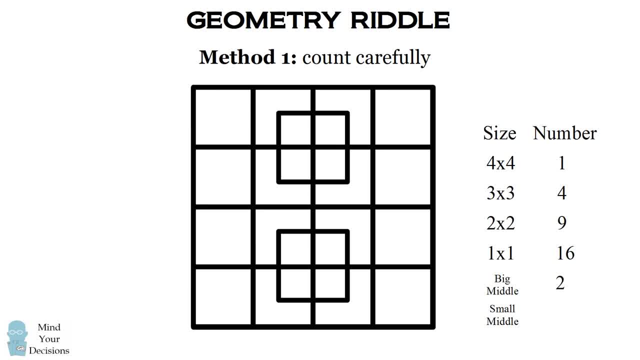 Each of these squares is going to contribute four more small squares, and there are two of these, so this will contribute eight more squares in total. We add up all of these numbers and we've counted that there are 40 squares in this picture. Did you figure it out? Now? there's a shortcut we could use if we're going to do problems like this. If you have an n by n grid, there will be one square. There will be one squared plus two squared, plus all the way up to n squared. number of squares: 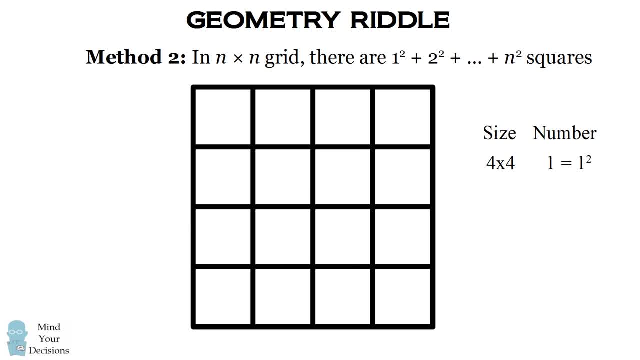 We found this already, that the number of four by four squares was one, which equals one squared. The number of three by three squares was four, which equals two squared. The number of two by two squares remember there were nine, because there were three squares per row and three rows. And the number of one by one squares was 16, because there were four per row and there were four rows. We could have started out by counting this without even doing the count of the squares, just using this formula, and then we would have had to add on the number of squares created. 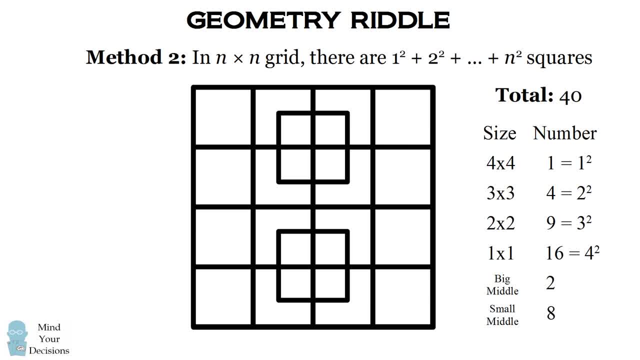 by the squares in the middle, which would have been 10, and that would have again got us to the answer 40. So you can intuitively see why this formula is true. You count the number of squares created per row and the number of rows you have. but let me just provide another proof. We'll use induction, So we'll assume the formula is true for n and we'll prove it's true for n plus one. So we have an n by n grid and we're going to add on one by one, squares on the side.